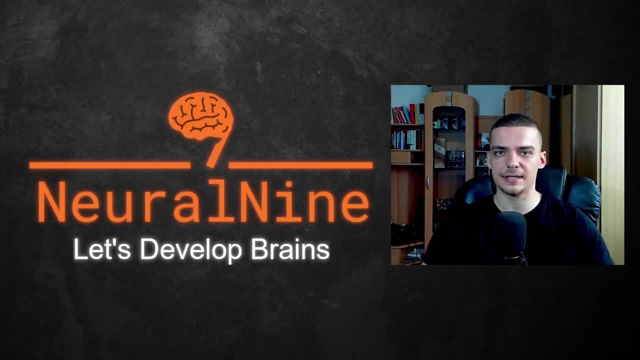 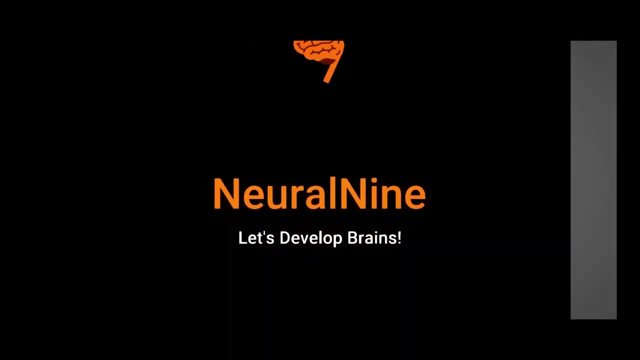 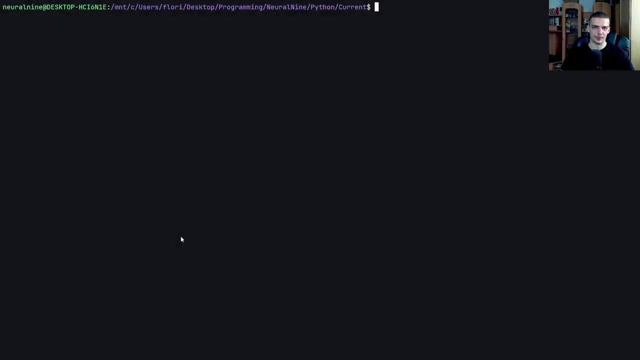 What is going on, guys? welcome back. and today's video we're going to learn how to properly import our own custom python modules into our scripts and also what the role of the init py files is in that context. so let us get right into it, All right? so today we're going to work with multiple files and multiple directories, and 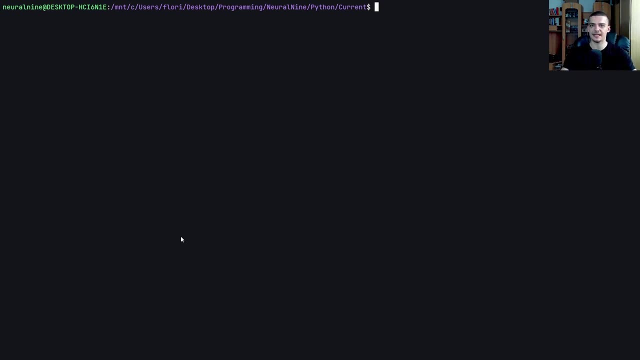 please don't be confused by my development environment. i'm using neovim inside of the windows subsystem for linux, so inside of a terminal on windows. but that is completely irrelevant to you. you can use whatever you want. you can use vs code, pycharm, notepad, plus, plus. 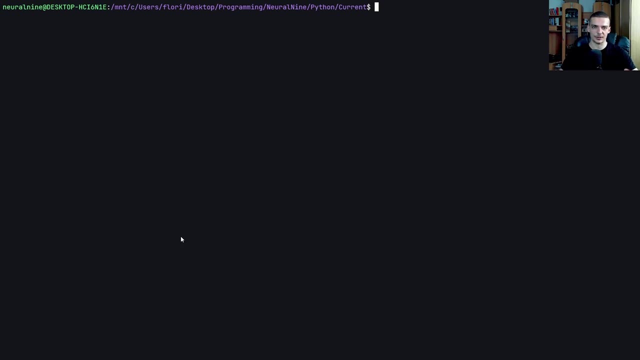 the python idle doesn't matter. all you need is a directory where you can create multiple python files and directories, and you need a python editor and a python uh development environment. that's basically it. you just need to be able to run python scripts. i'm going to use this environment. 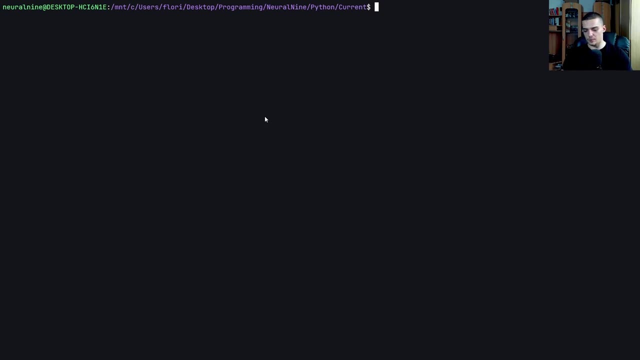 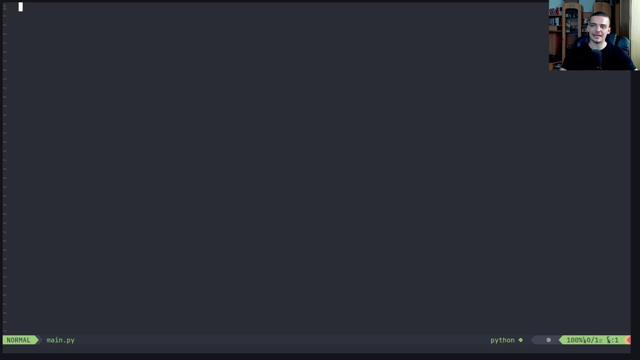 but don't be confused by that. so the first thing you want to do is we want to create a file called mainpy, and this is going to be obviously our main file. here we're going to run code, and the goal is now to have functionality in different python files that we can then import into the 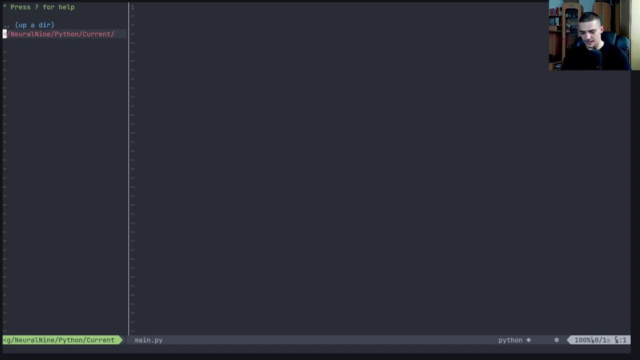 main file. so, for example, let's create a second file here. let's say we have um a file. i'm going to call it functionalitypy. we just create this file here, um, and essentially we're going to open this now in split mode. here i'm gonna just define a couple of arithmetic functions. so i'm gonna say: 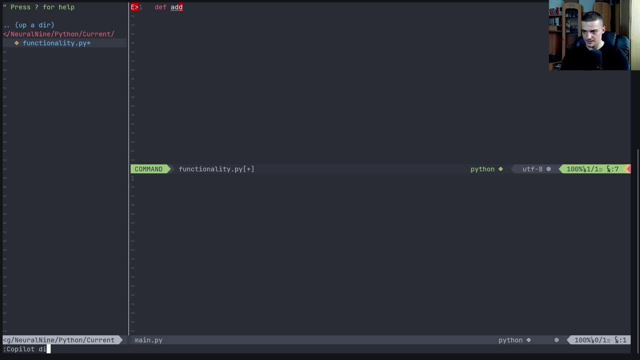 add. now let me just briefly, before it fires up again, disable the auto completion. so we're gonna have add taking parameters x and y, returning x plus y, very simple functions, and we're gonna copy this now and we're gonna have the same function here for sup. we're gonna have the same function. 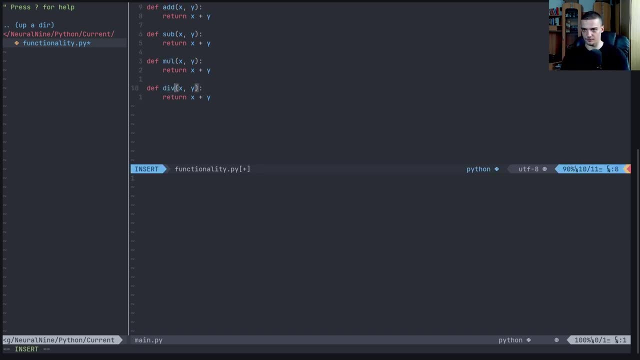 for mul and we're gonna have the same function for diff and we're gonna change the respective operators here. so those are the functions that we would like to use in the main file. how can we do that now, when we have just one file? this is kind of simple. all we need to do is we need to say, uh, from functionality import, and then i can. 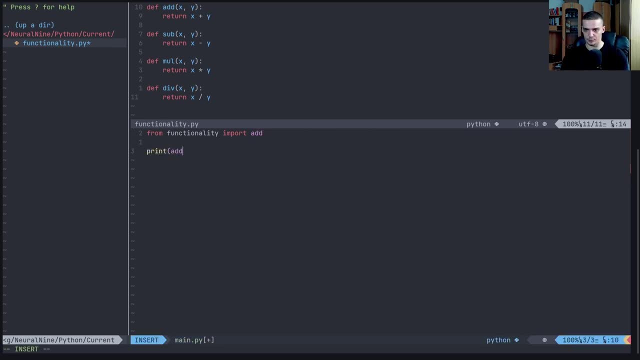 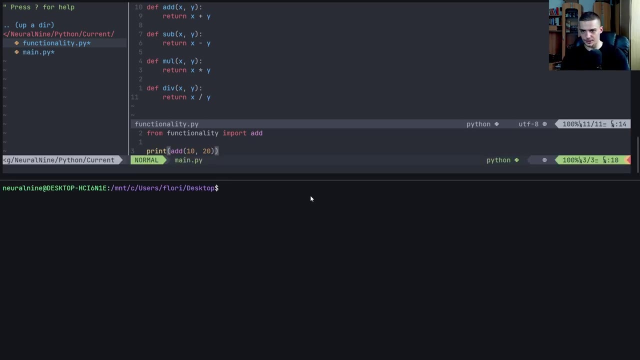 say, for example, add, then i can print print at 10 and 20.. so that's quite simple. um, i can now open up a terminal here. i navigate to the directory that i'm working in and i can now run the python. don't be confused by the environment. all i did is i created two python files in the same directory. 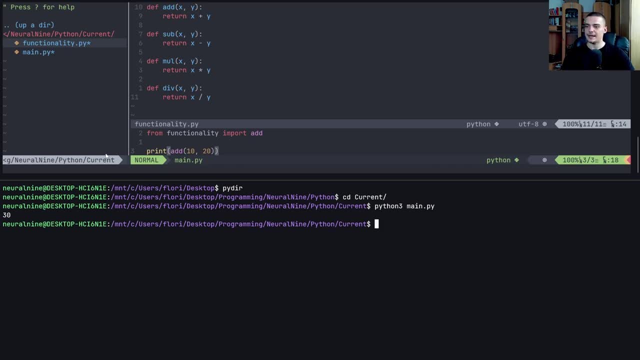 and i ran them in the terminal, so you can do that as well. um, and you can see it worked. so now i used the add function of the functionality python uh file and i used it in the main file without having the function defined in the main file, by just saying from functionality, import at. so this is. 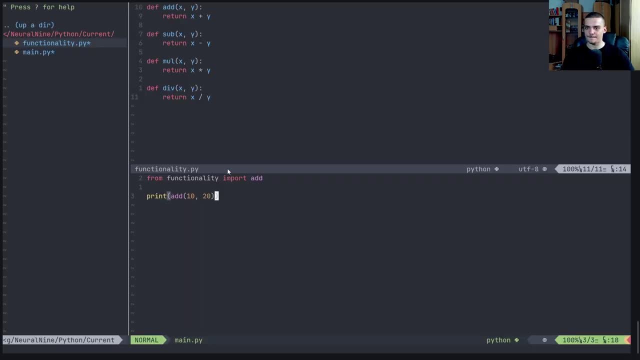 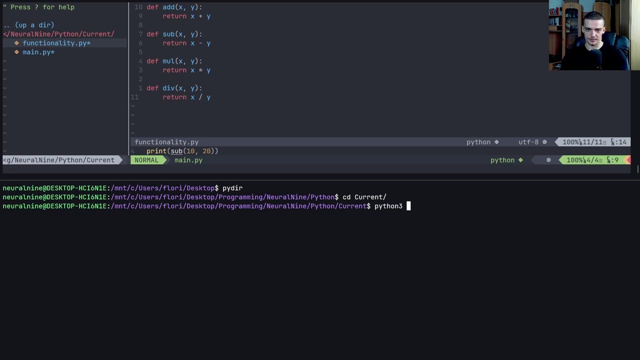 kind of simple, nothing too complicated here. um, now, what i can also do is i can say from functionality import add, and then i can also use add, and i can also use uh, sup and let's see if that works. python3 main py, you can see it works without problems. um, so that is how you do that. if you 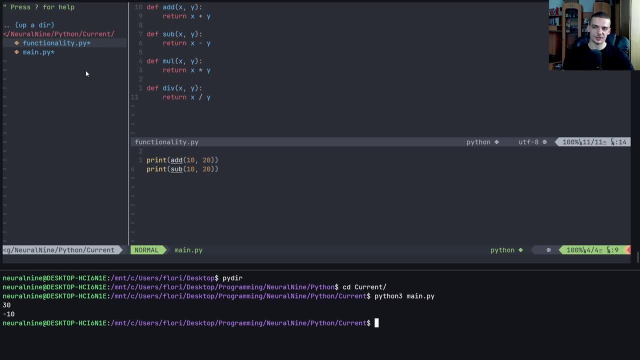 just have a file in the same directory. now let's say you don't have just a single file, but you have an actual module. so you actually have a directory with multiple python files that have different functionality. uh, in those files. so let's say, here i'm going to create 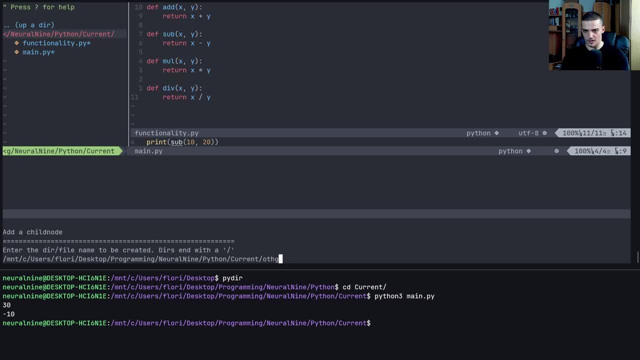 now a new directory- let's call it other module, and inside of that i'm going to create a python file called second dot py. i don't know, just just some file here. and let's open this file and let's say we have a function, my function, here, and let's say i just want to print hello. 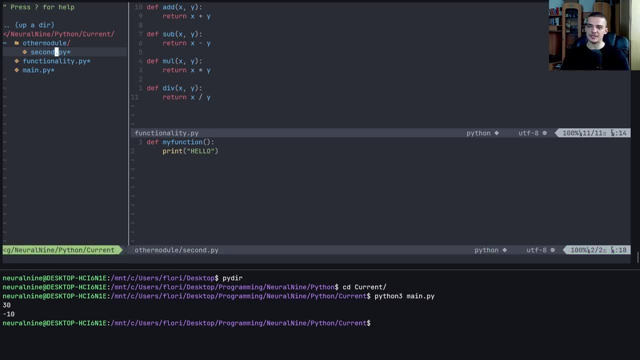 with this function. so in order to use this function now, i don't have to do anything fancy. i just go again to my main file. i say from, and in this case other module, import, and um, i can just import here now the second. so the difference here is that i'm importing. 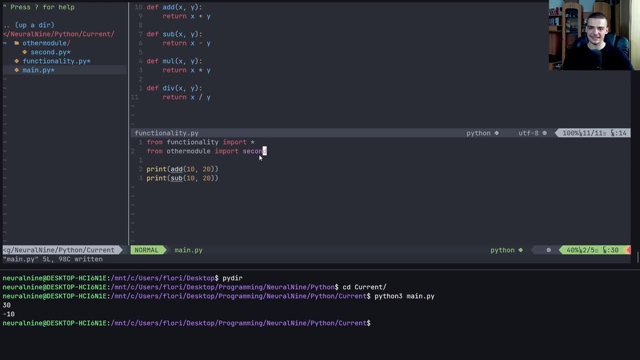 now the full file. so if i have multiple functions, this is not a function. here i'm saying: from the file functionality, import the different functions, whereas here i'm saying from the module, from the directory, other module, import one of the python files. and if i now want to access the 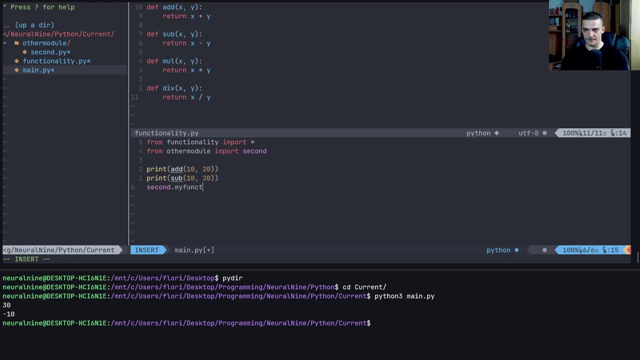 function, I have to say second dot my function, like this, in order to execute it, in order to call it. or, of course, alternatively, I could also say import. or actually I can say from other module dot, second import, everything, And then I could just run, I could just call the. 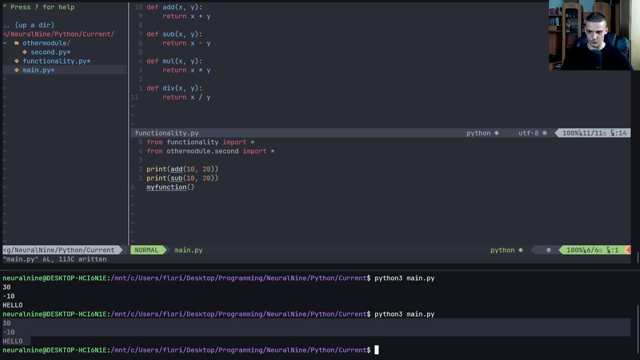 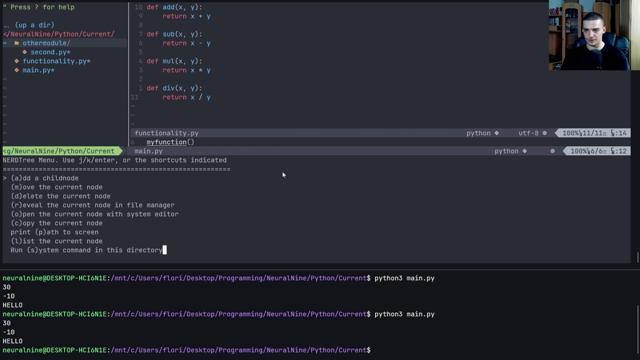 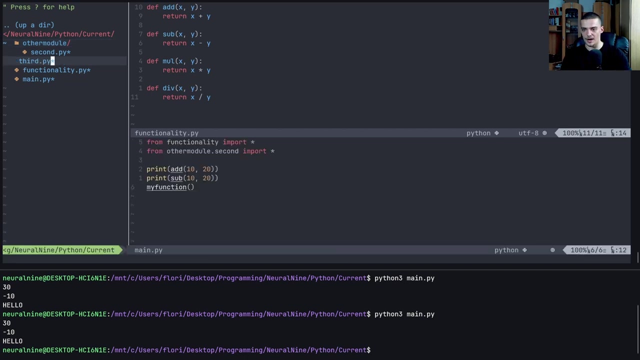 function without referring to second specifically. So that works as well. The interesting thing now is what if we have multiple files- and this is maybe something new to you, because that's up until now this was actually quite clear- Let's say, I have another file here, third, dot py And. 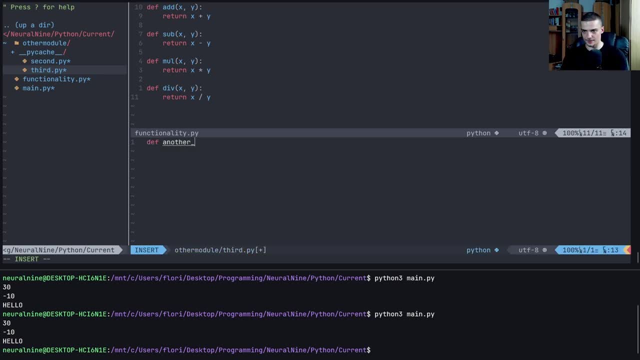 I have I don't know another function, And this time it prints ABC or something like that. And now let's say I want to do something else, I want to go into my main file and I want to say: from other module. 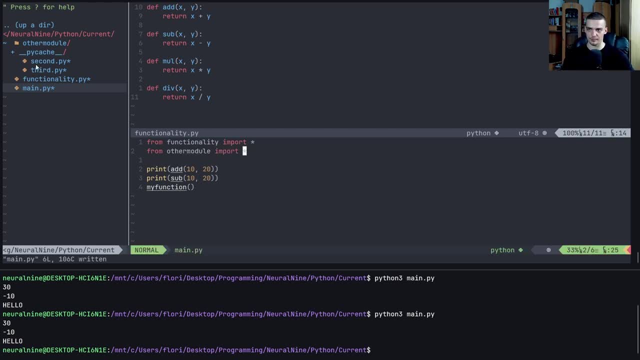 import absolutely everything. So I want to import second and third And I want to be able to do something like second dot my function. How do we do that? Because if I try to do it like this, if I just say from other module, import everything, and I want to import those two files. 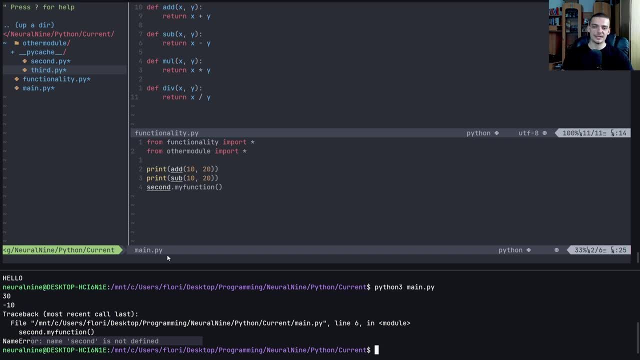 you can see it doesn't work. And this now is why we need the so called init py file. So underscore, underscore, init, underscore, underscore py files that you see in so many projects that you've seen it's auto automatically created. in PyCharm, for example, this file has the functionality to: 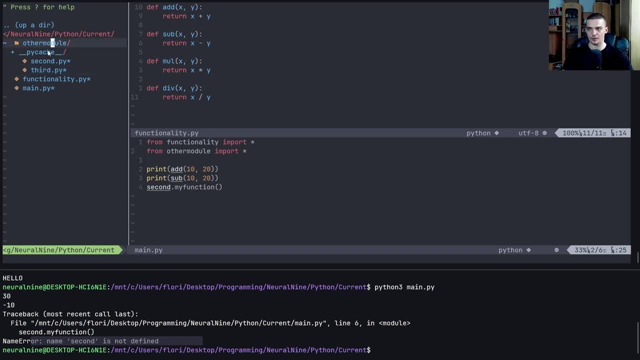 actually make a directory into a module. So if I go here to other module and I create this file, so underscore- underscore- init. underscore- underscore- dot- py, If I just create it, this now makes this directory to a module. So now this is recognized as a module And inside of this, 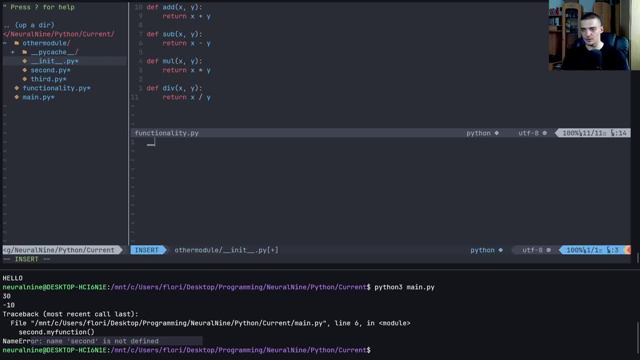 file. I can also write the following line: I can say underscore, underscore, all underscore underscore equals. and then I can provide a list with strings, And these strings refer to the file name. So I can say here, second and third, And now this, already this file, here this init py file with this line: 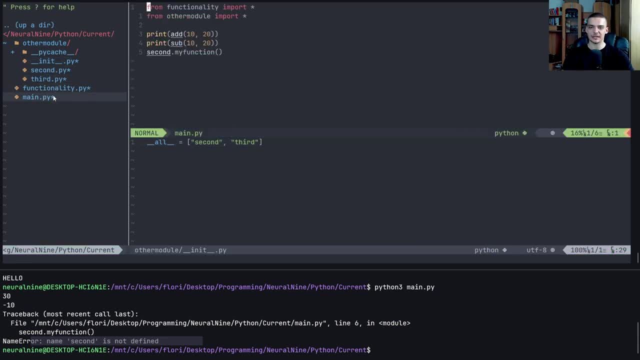 of code being in the same directory as those two files. this will allow me to use this notation from other module, import star, because what happens here is the stars decoded into second and third, And if I now run this, you can see this works. 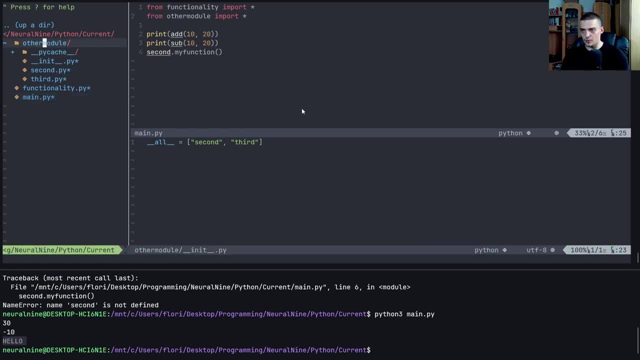 So this is how that works. Another thing of course is you can go ahead and create a sub module. So I can create another directory sub module, for example inside of other module, And here I can create a file- let's call it fourth dot py, And if I open it and I say last function, print I. 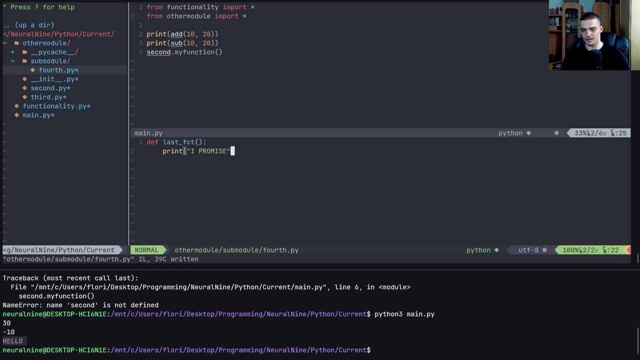 promise, There you go. Now I can go into my main main file And say: from other module dot, sub module, import, for example fourth. So this should work. I think if I now say fourth dot, last function like this: This works, as you can see, and I think it should. 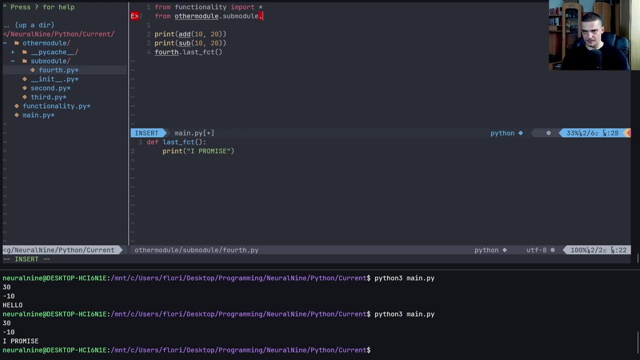 also be possible to say dot fourth import, and then last FCT. then we don't have to use the fourth. So, as you can see, this works as well. Now, one last thing that I want to show you is a notation. I'm not sure if we actually need it. 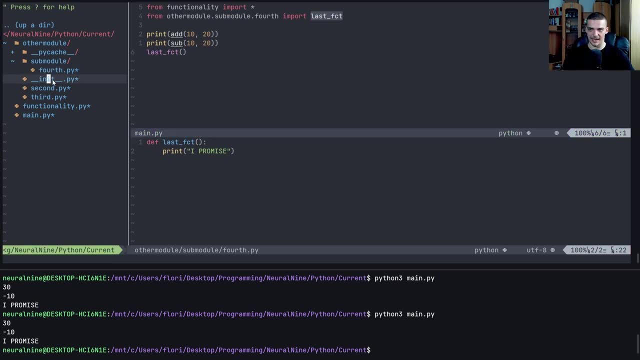 anymore. But one thing at least: to make it backward compatible, compatible. And if you publish your own package- this is also always a good thing to do- You can also write the import statements, for example, of the respective module here inside of the end up y file for clarity. So you can say from dot. 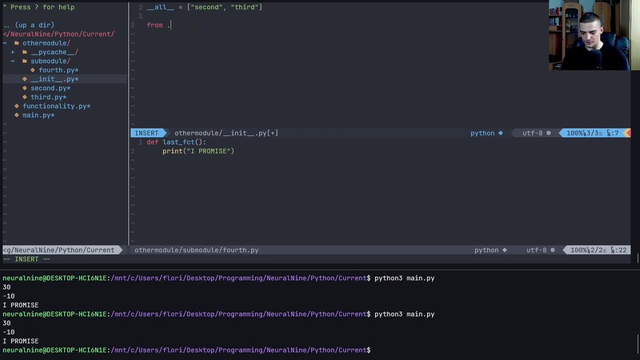 another, not another. sorry, this is my prepared code From the dot. second, we want to import. what did we have here? my function, So my function. and from third, import another function was the name, I think. So this is how this is done professionally.